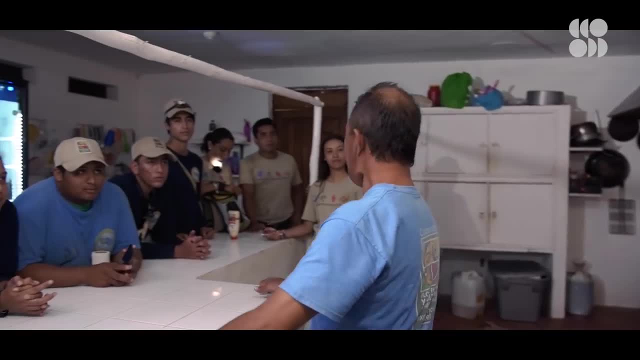 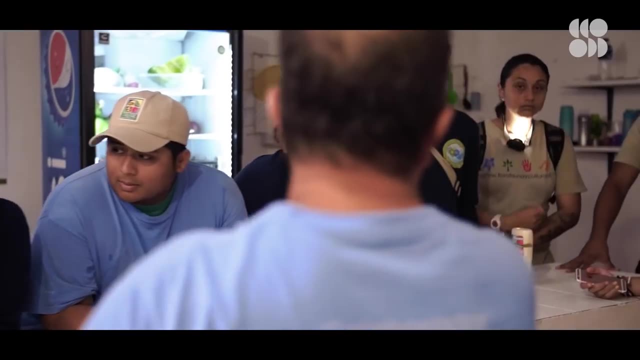 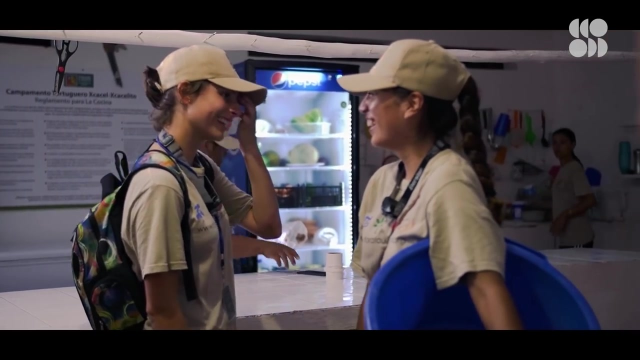 Bye, Bye. At the camp, we patrol the beaches every night in the search of sea turtles that come to nest, so we can have an accurate record of all the specimens that come to Xcacel each year. You can be burned out, but being surrounded by everyone getting ready somehow lifts your spirits. 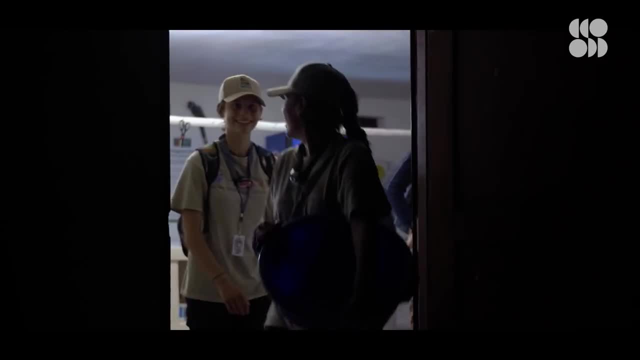 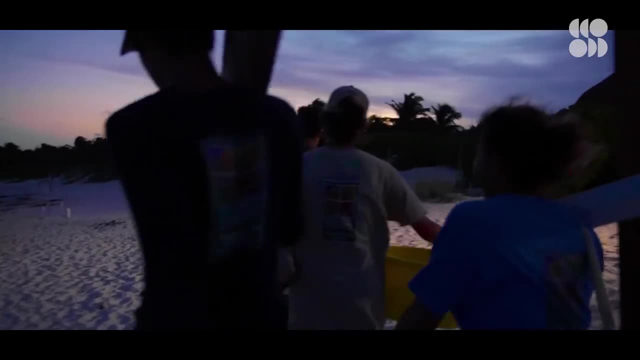 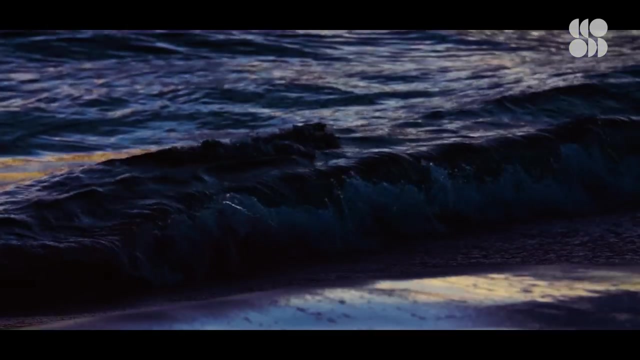 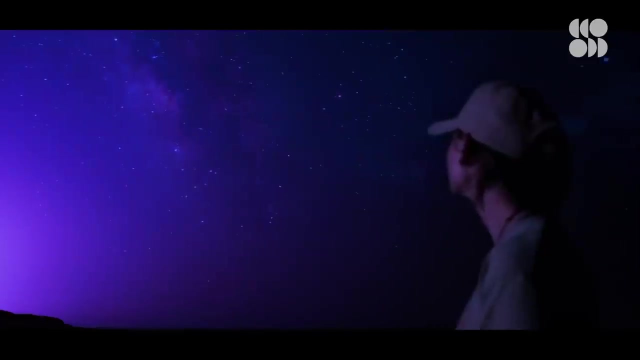 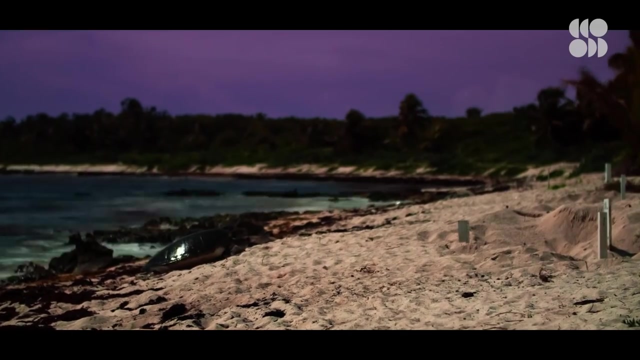 You walk through the beach, feeling the sand on your feet, the wind in your face, hoping for it to be a windy night that keeps the mosquitoes away. You feel connected to the sea, the stars, and wait for the first sea turtles of the night to appear. 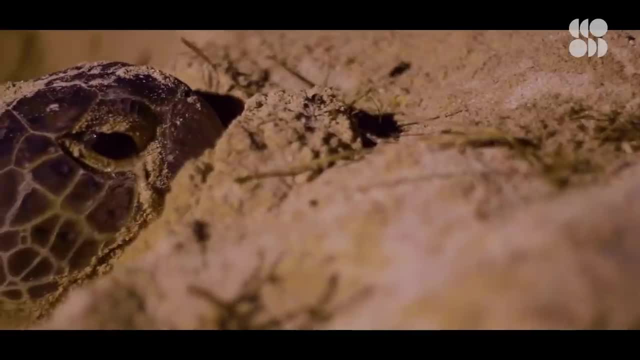 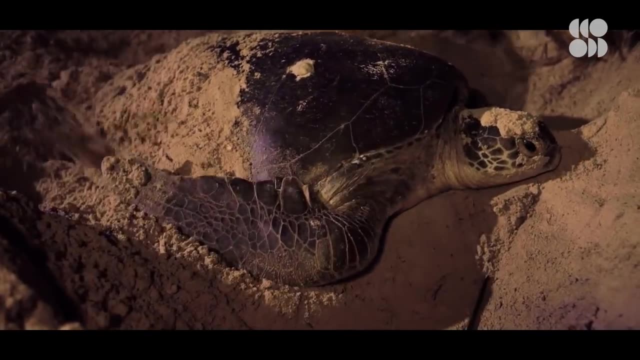 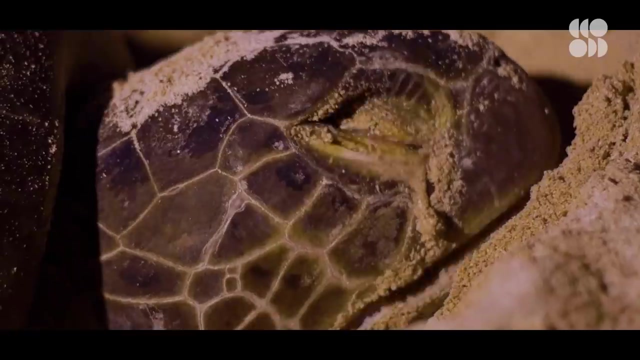 Loggerhead and green sea turtles come to the shores of Xcacel to nest both endangered species. Some can take over two hours nesting and can lay more than 120 eggs. The immense effort forces them to stop constantly, but only to take a deep breath. 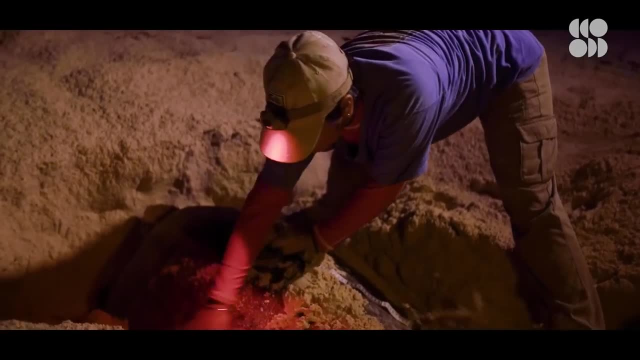 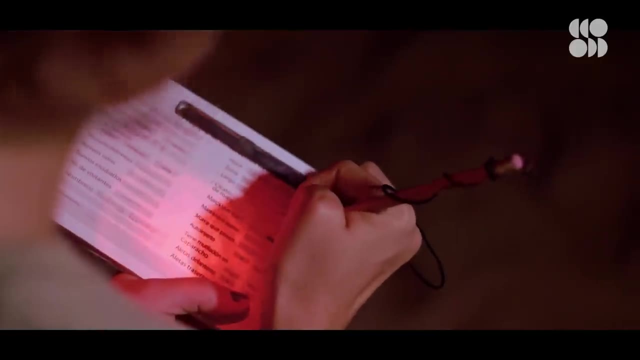 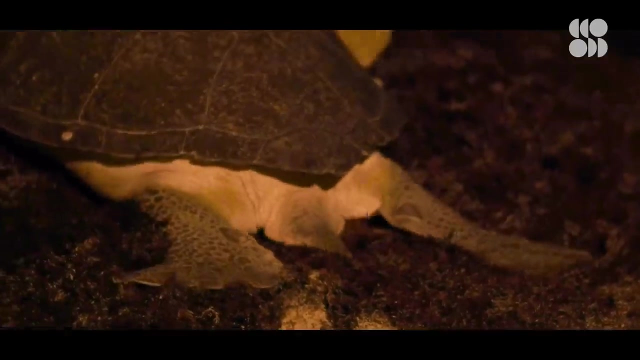 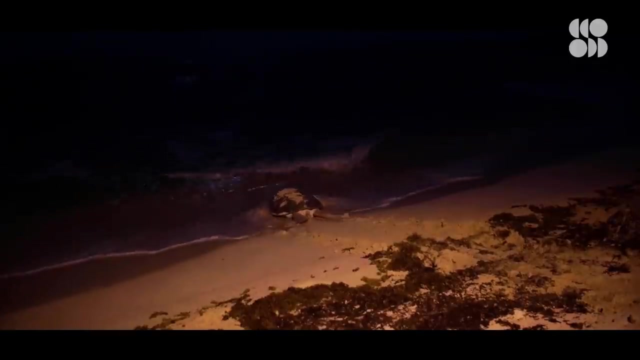 and carry on with the termination. We don't just take measurements, We also protect them from any adverse situation that could happen along the way. To witness how they end in these beaches such a long and rough journey always leaves me in awe. They're completely free. They go wherever they want through the vast ocean. 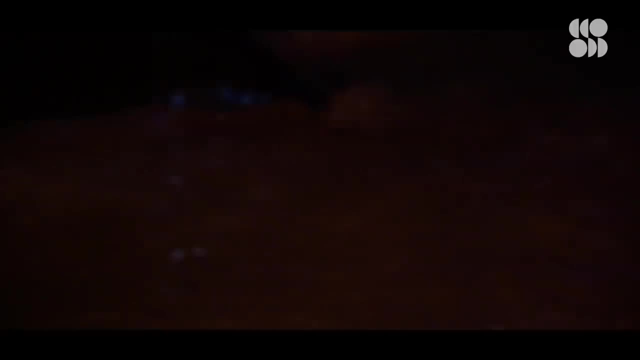 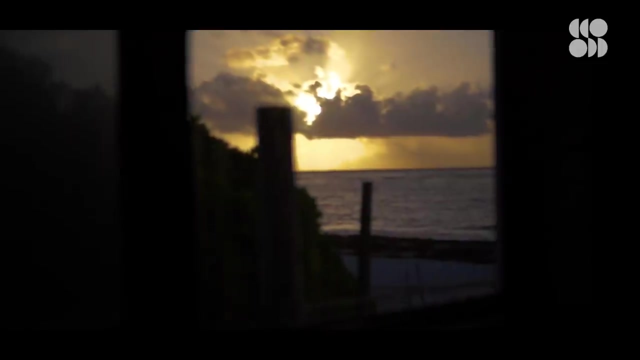 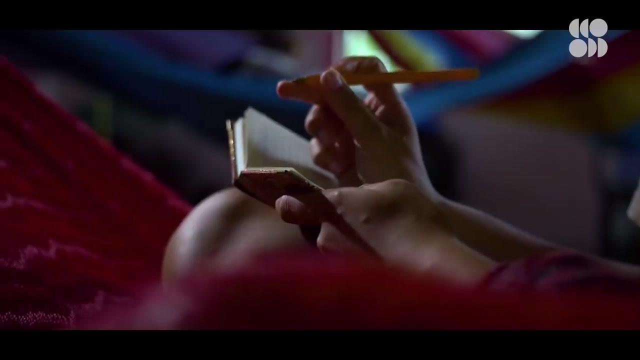 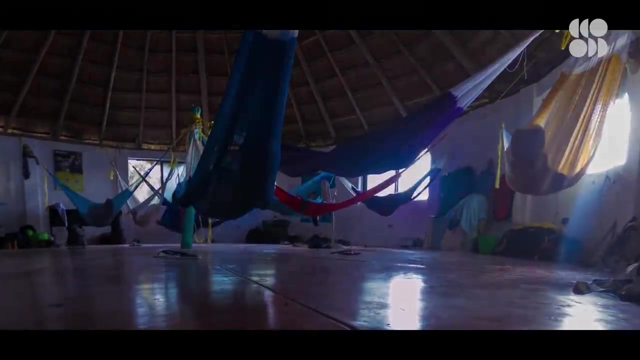 However, they always come back. They never leave. They never leave, never forget their home. to be part of this program, you have to be able to adapt, sleep little, have odd schedules, but it's easier when you're a company. we're volunteers of all ages and all parts of Mexico who have come together. 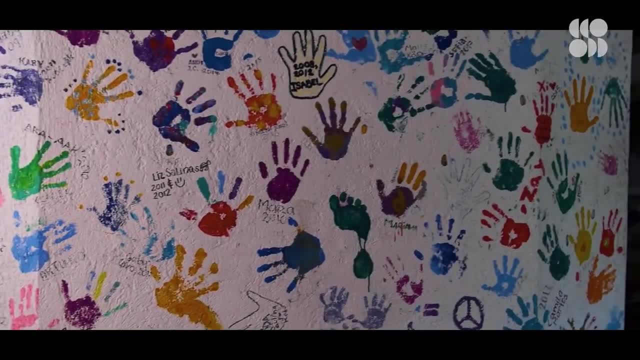 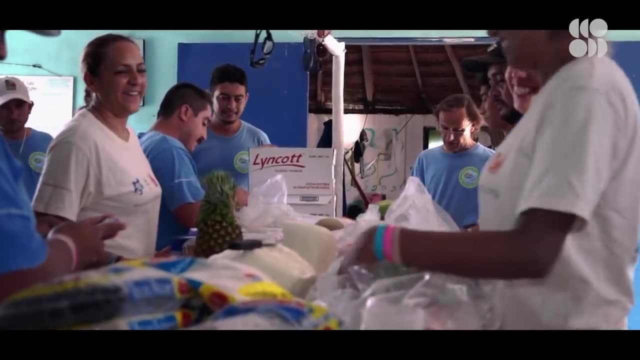 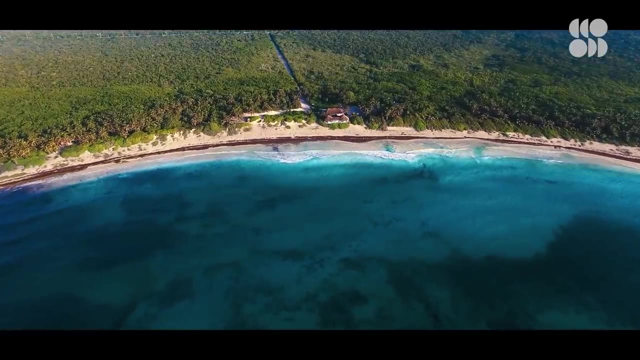 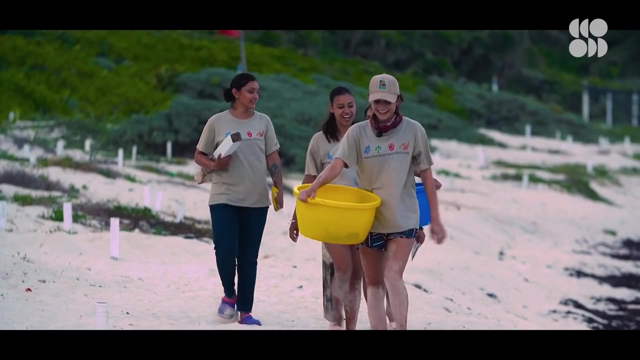 to put all our energy in the protection of this natural sanctuary. Scassell is a very attractive place for tourism and even though it's a natural protected area, it is constantly endangered by resorts and real estate firms. that's why this is a great place to stay. 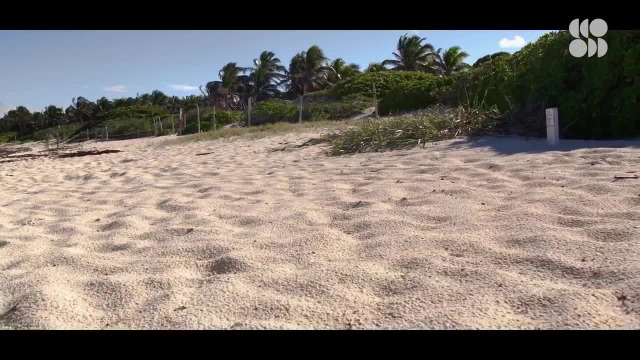 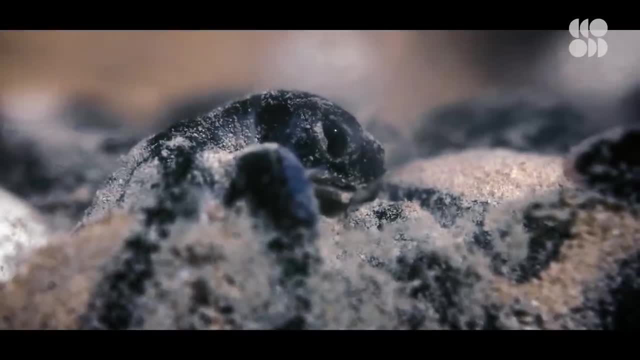 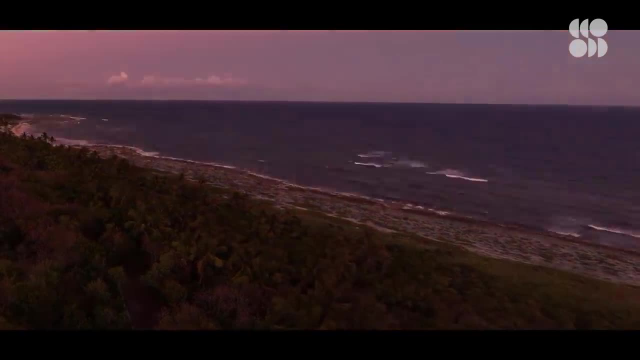 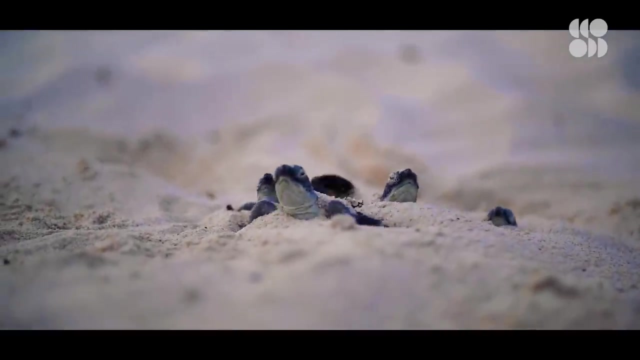 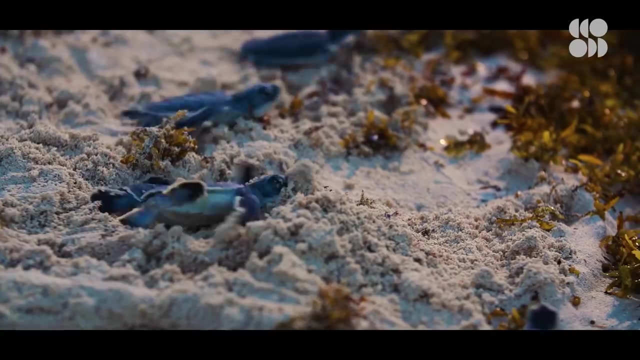 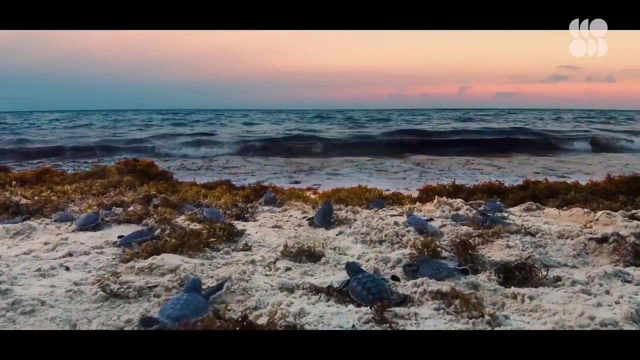 this conservation project is so important. at dusk, when frigate birds leave, the newborn sea turtles can hatch safely. on one side, the immensity, on the other, the tenderness of the newborn sea turtles going towards the sea. it's incredible to see how it all coexists in 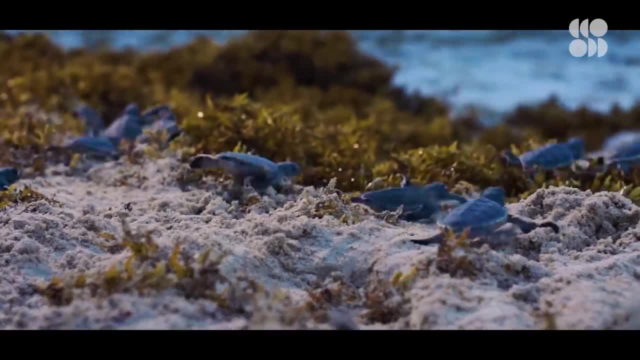 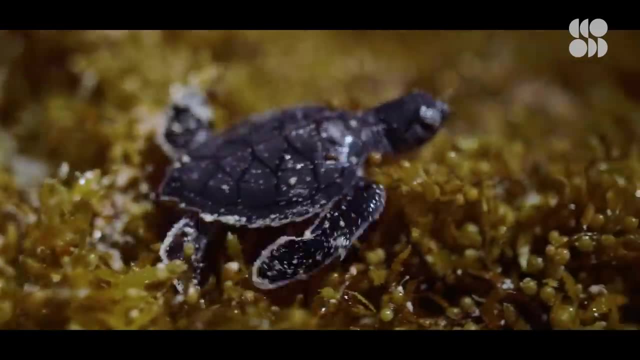 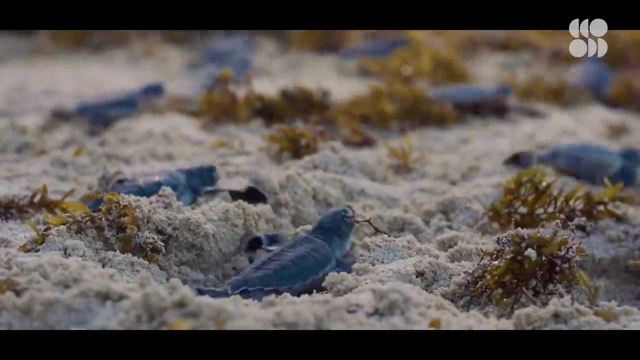 the same space. for every thousand sea turtles that cross the beach, only one will come back as an adult, but that doesn't stop them. they just hatched, they're new in this world and they go straight to adventure, to the toughest and wildest places in the world. 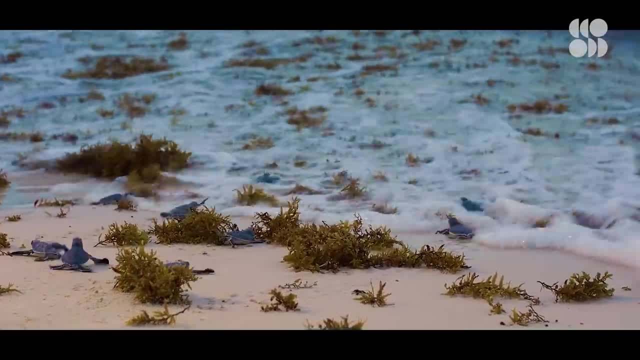 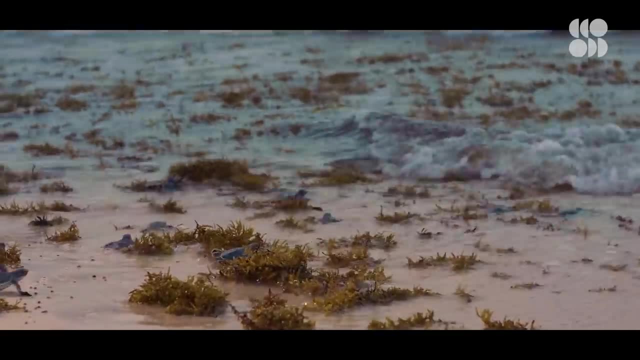 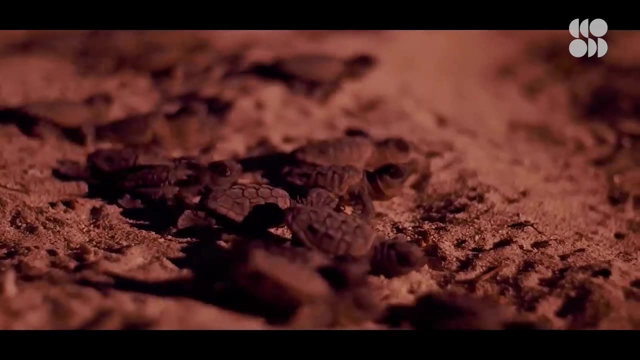 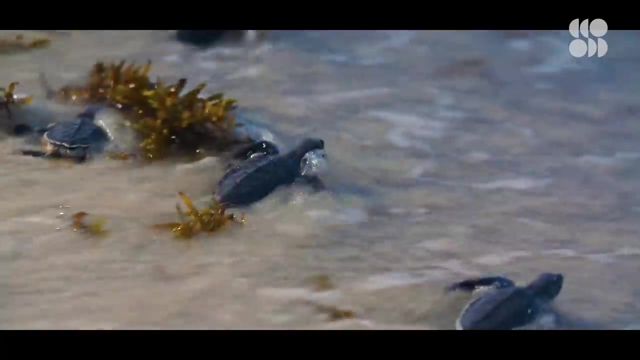 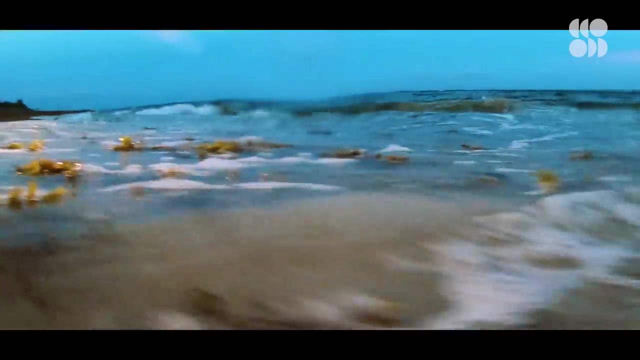 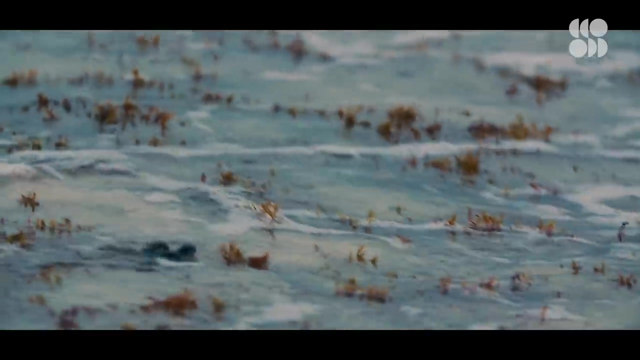 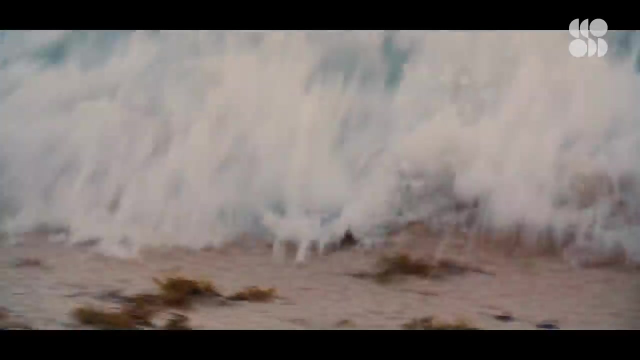 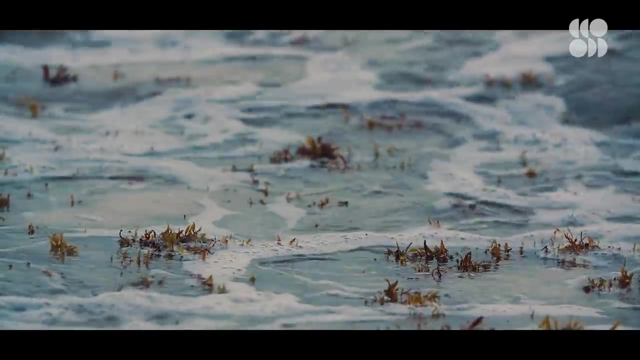 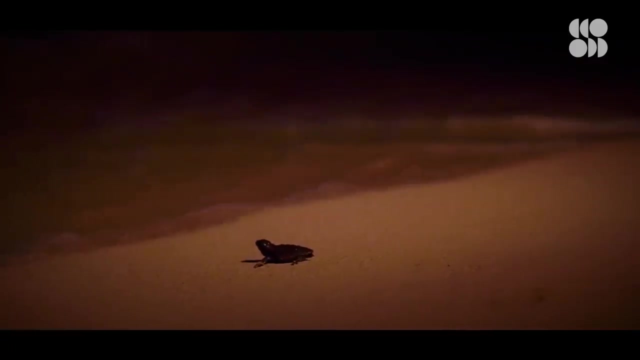